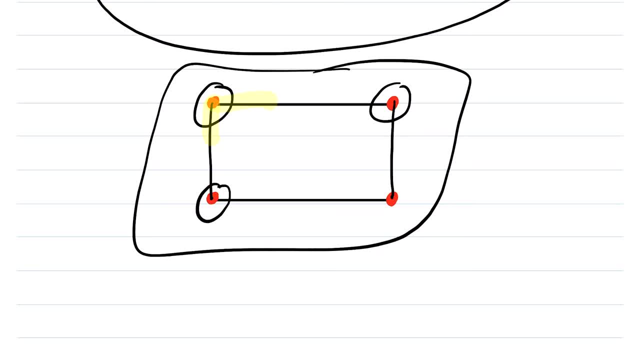 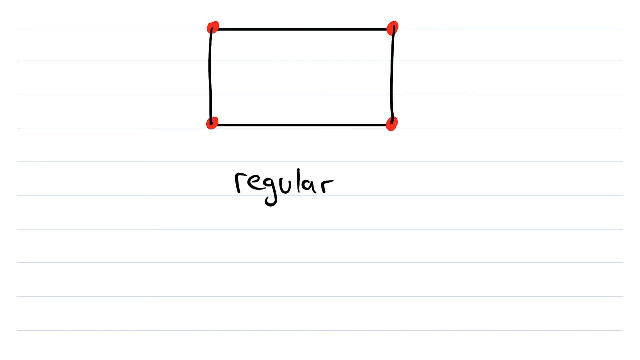 and every vertex in this graph is adjacent to two vertices, so it is a regular graph. So this graph is regular, like we've been saying, because every vertex has this degree one and when I actually switch it to a helping hand, it is very easy to understand. 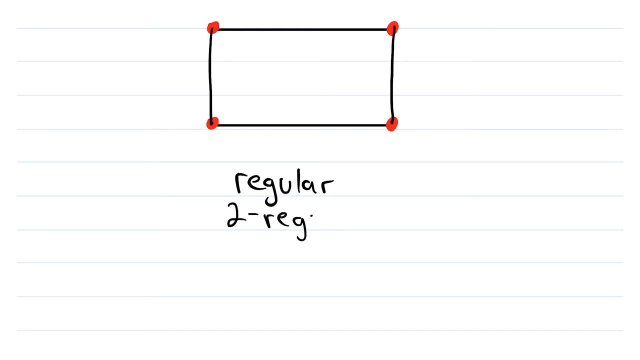 this one, because if you open every vertex in this graph, there's probably a few vertices that are adjacent to both and it's just represented by this one event. This is a regular, so let's a regular. help you. yeah, and same degree. it is also too regular. to get more specific, we say that it is too. 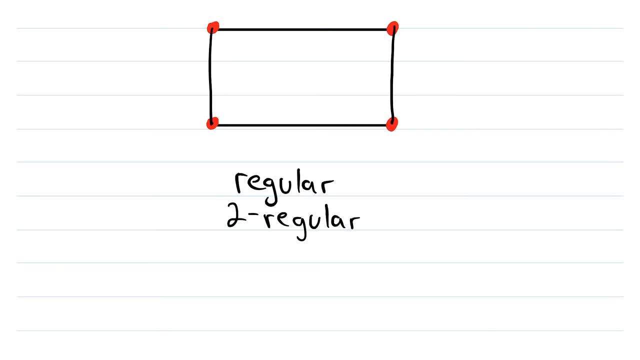 regular because every vertex has degree 2. and then, lastly, if you want to call this graph more names, you can say that this graph is regular of degree 2, of course, again, because every vertex in the graph has degree 2. so we can say it is a. 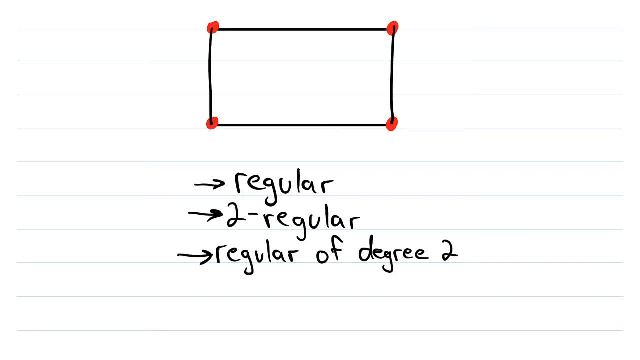 regular graph. it's too regular. it is regular of degree 2. now how about a 3 regular graph? that would be cool, the thing we can find. one of those. we absolutely can check it out. just have to join these two vertices here and join these two vertices here with that super straight line there. so this graph is 3. 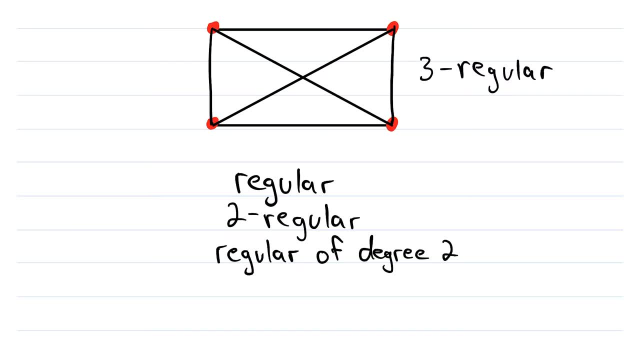 regular because every vertex in the graph has degree 3. looking at this bottom left vertex, for example, it's incident to one, two, three edges and equivalently it's adjacent to one, two, three vertices. you now, if a graph is 3 regular, we can also say that the graph is cubic. so a 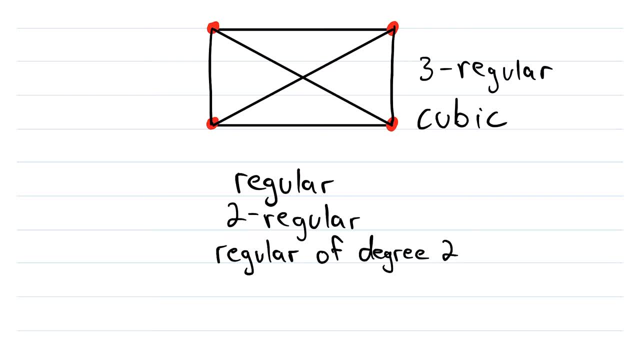 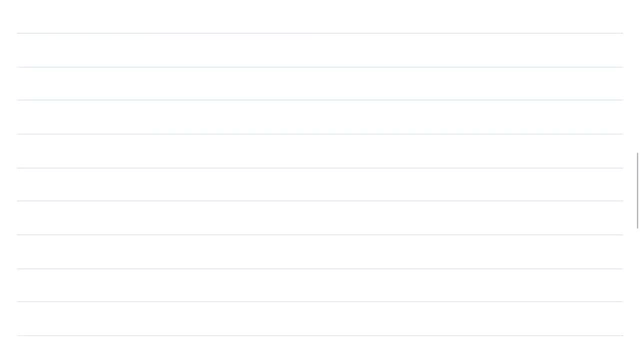 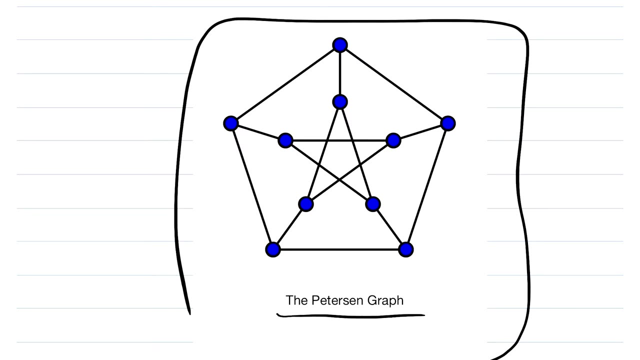 cubic graph is a graph that is 3 regular. any graph where all of its vertices have degree 3 is a cubic graph, and scrolling way on down here, this is the most famous cubic graph. this is the Peterson graph, as the caption says, and I got this. 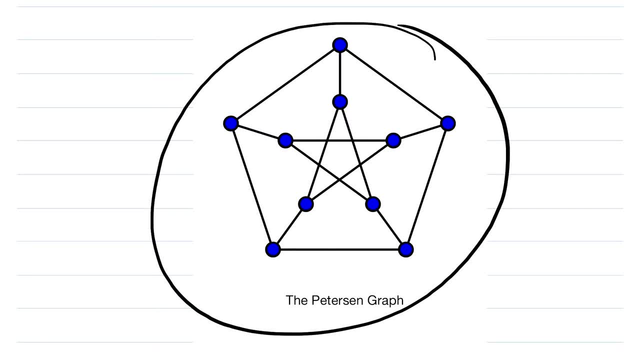 picture from Wikipedia, just so that we could see a perfectly drawn Peterson graph. like I said, this graph is cubic and it's quite a neat looking graph. so again, it's cubic because every vertex has degree 3. let's look at a couple. this vertex over here, for example, is adjacent to one, two, three vertices. so indeed it.